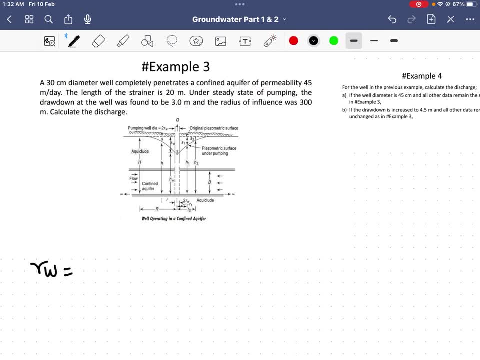 informations. so i have the rw. so rw means i have to divide my diameter by two. so i have 30 meter diameter. so i will divide it by two, i will get 15 centimeter. so if i want to convert this 15 centimeter, i have to make meter. so i will get. 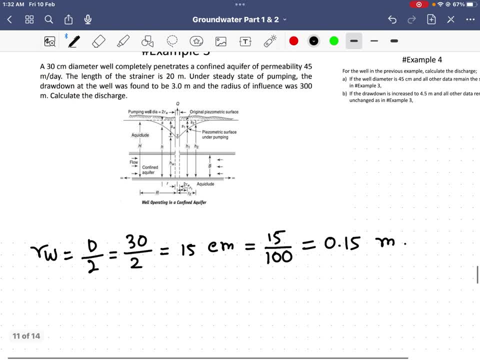 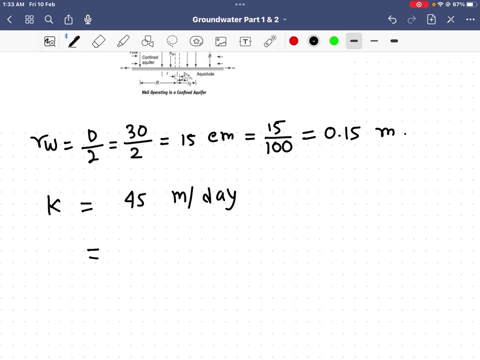 0.15 meter. simple, then i will get my another information. i already have the permeability, so my permeability is k. right, so k equal 44 meter per day. okay, so i have my permeability in meter per day, but i want to make it meter per. 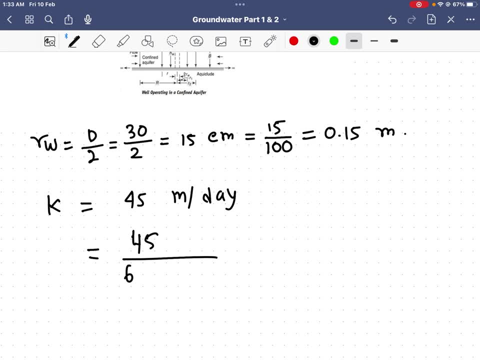 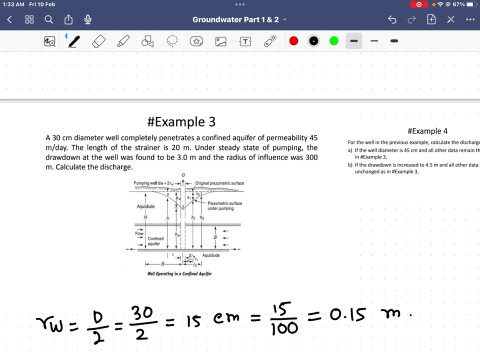 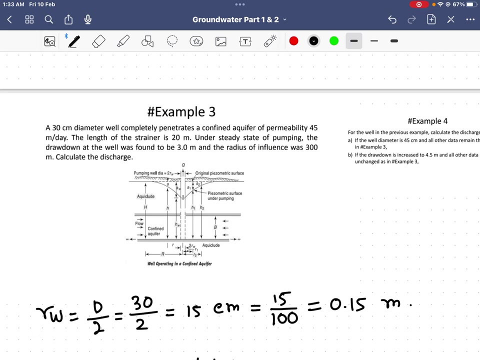 second. so 45 times day, 60, 60, 24. if i do, i will get 5.208 times 10 power negative 4. this is meter per second. all right, so now. now i will read this: the length of the strainer is 20 meter, that's mean the b equal 20 meter here. all right now, under steady state. so my condition: 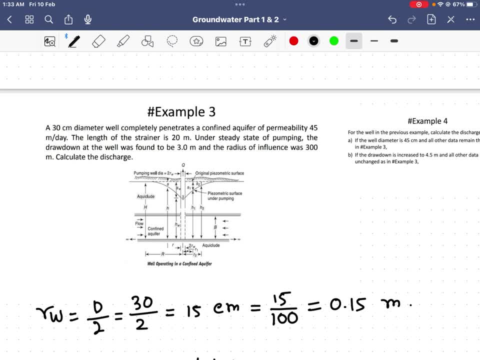 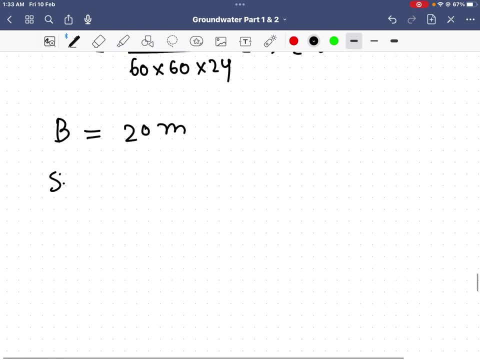 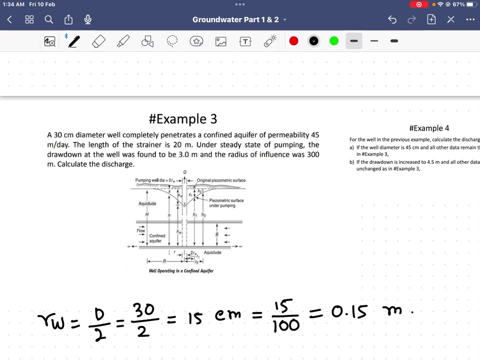 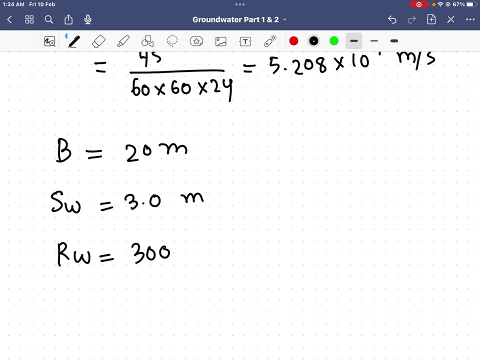 is steady state. the drawn drawdown at the well was found to be three meter, so my sw is equal three meter. okay, so now the radius of influence. so i have the radius of influence, which is called rw, so which is 300. all right, so all the informations that 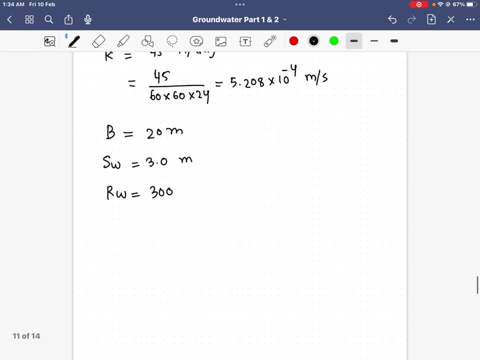 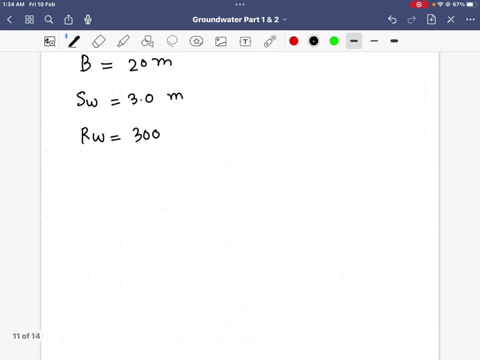 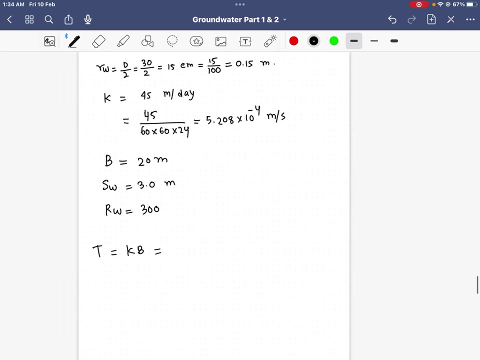 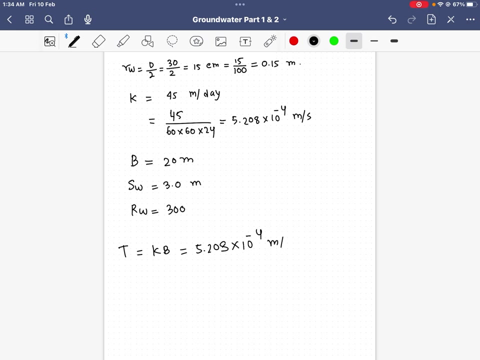 available in my questions. i already list down in my paper. all right, so now once i have the k and i have the b, so easily i will get the transmissibility. so t equal kb. so i will write down my k value. so my k value is 5.208 multiplied 10 power negative 4 meter per second times b. 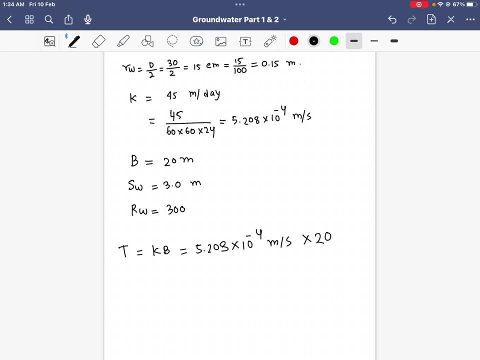 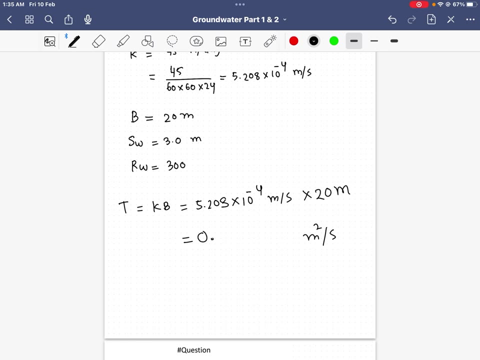 my b is 20 meter. all right, so i will get this meter, and meter will be meter square per second, then 5.2. if i multiply it will going to be 0.010416, so 0. i can write in this way also: 0.10, 10.416 times 10 power negative 3 meter square. 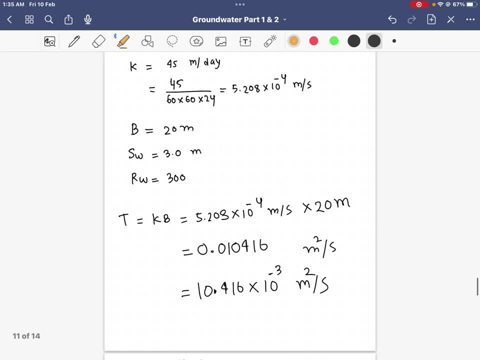 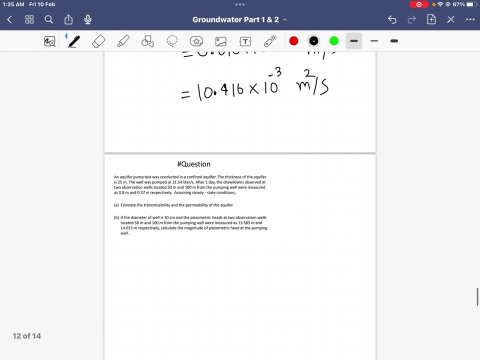 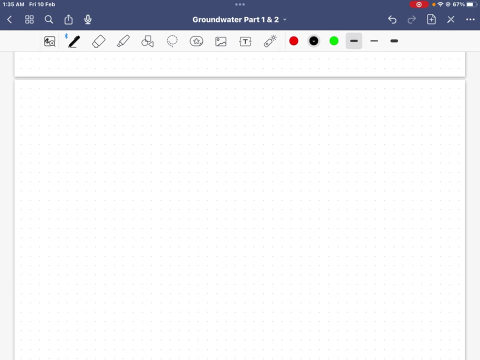 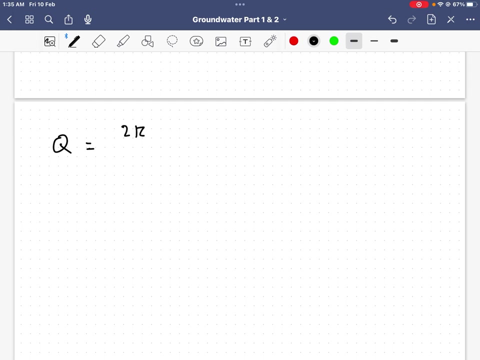 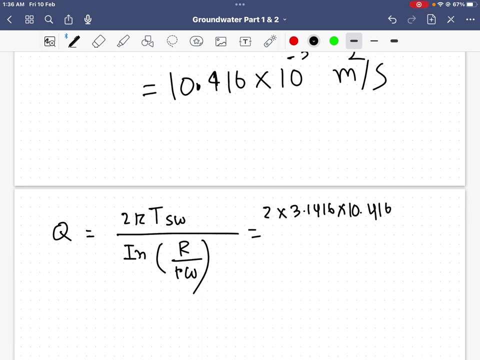 per second. so i already get the transmissibility t. okay, so now let me take one page. all right now i have to find out the discharge q. okay, so we have the formula 2, pi t, s, w divided long r over r w. okay, so i have 2, 3.1416 times. i have the transmissibility 10.416 times 10 power. 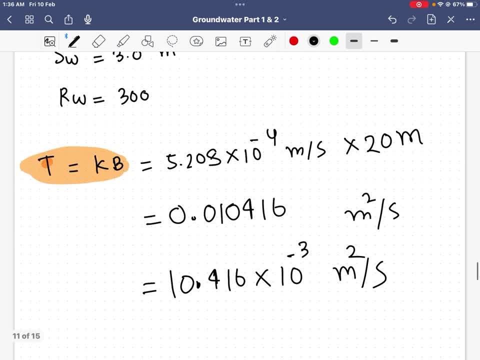 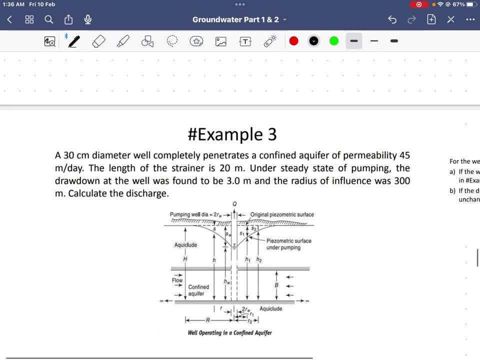 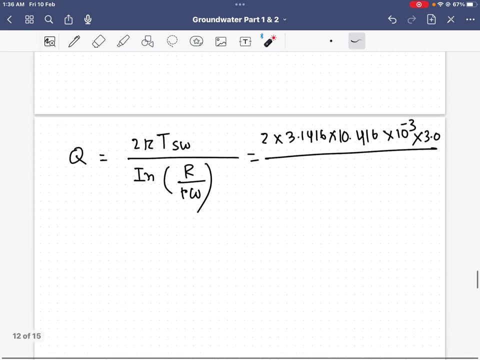 negative 3 times. i have also sw, so sw equal 3 meter. okay, because this 3 meter comes from here. you see, the well was found, 3 meter. okay, now long my r radius, influence, radius of influence. so i have 300 and rw i already got from the diameter 0.15. if i calculate i will get 0.02583 meter cube per second. 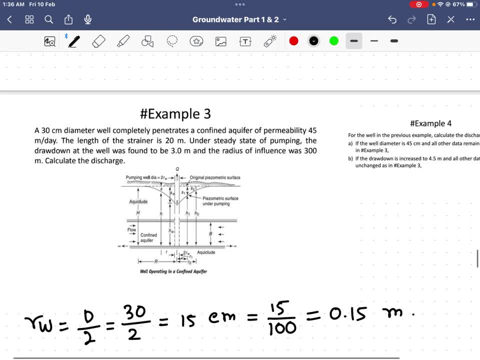 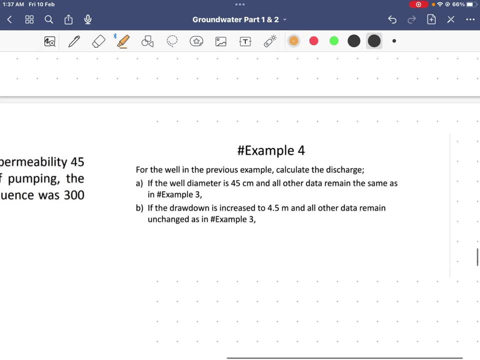 all right. so now i will get my exercise three finish, because i already find out the discharge. so now i am going to solve the example four. okay, in the example four, for the well in the previous example, calculate the discharge. so if the well diameter is 45 centimeter, okay. so now they change only the well diameter, okay. 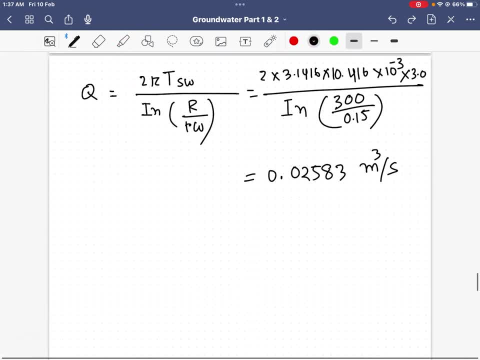 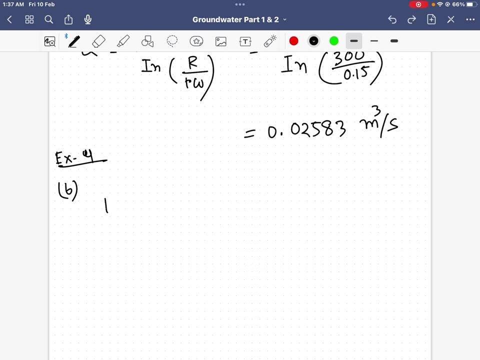 well, diameter. so if you see i can quickly, i can do these questions. so b example 4, i will get. so b equal. so i have, only i will change the diameter. so and all the value will remain. so rw equal 45 centimeter. so i divide it by 2. if i do divide it 45 over 2, i will get 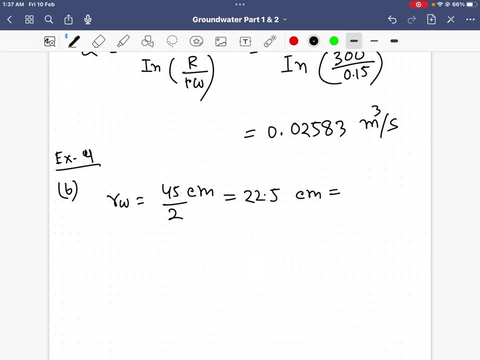 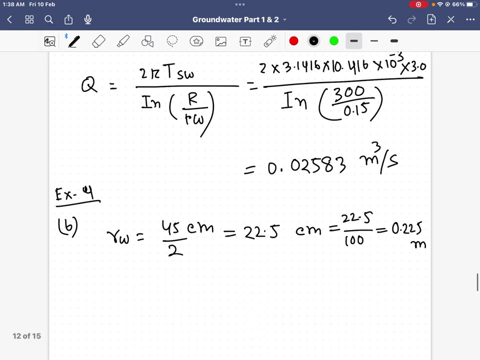 22.5 centimeter. so if i do 25 centimeter, 100 uh, 22.5 over 100, i will get 0.225 meter. all right. so if i want to get the discharge with the different uh diameter, but all the value is remain the same, 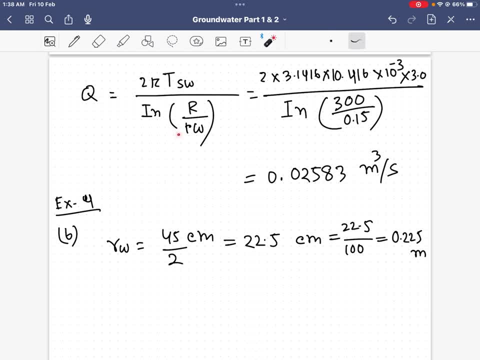 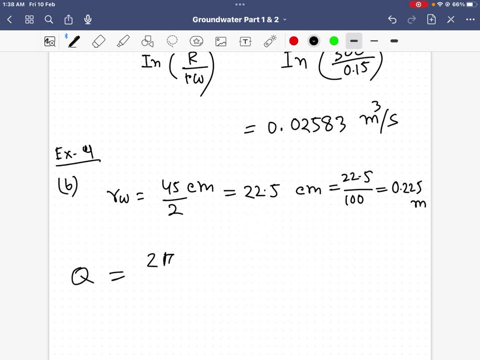 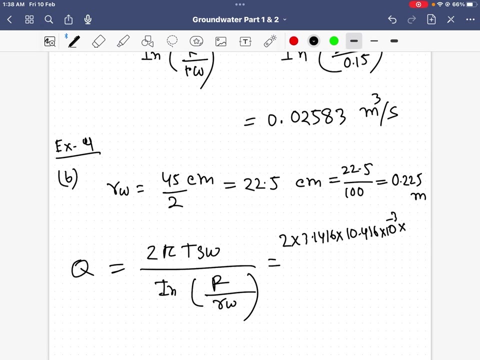 so i just change this part. okay, i just change this part. so q equal. i have the formula 2: pi t, s, w divided long r, influence radius and rw. so i will get 2 times 3.1416 times 10.4. one six times 10 power negative f. three times sw equal. three divided long radius, influence radius. 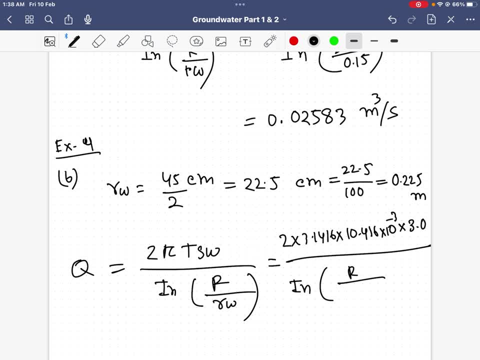 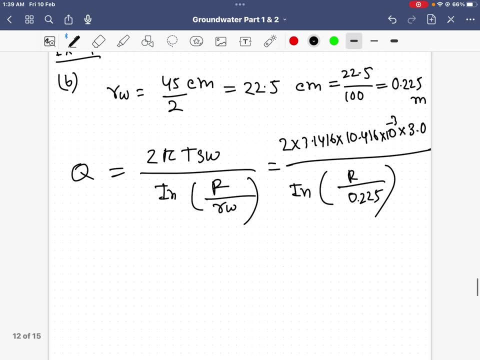 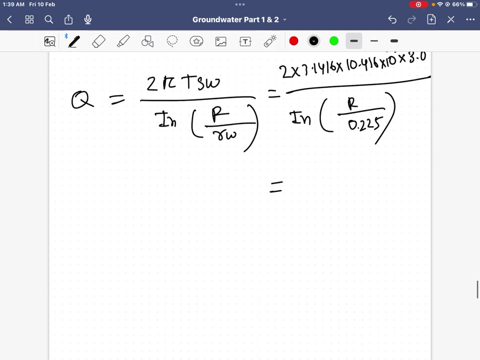 will be same, then i only will change the diameter. so my diameter in this case, if i do 0.225 and if i calculate it. so let me calculate two point three, point one, four, one, six times ten, point four, one, six times ten. power negative three: ten power negative three, then i will times with three. 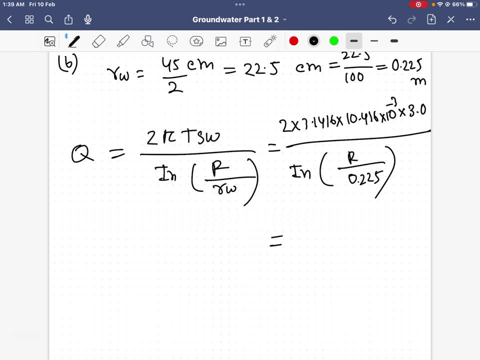 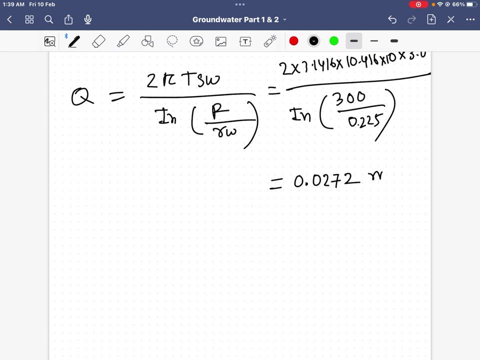 divided long. okay, so i will get three thousand and zero point two two five. okay, so i will get zero point zero two, seven two. let me get 0.0272. okay, so i will get 0.0272, and let me write this a means alpha. wanna also write an equal to or equal to.